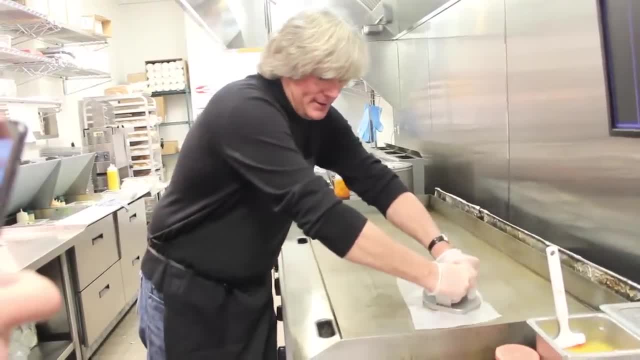 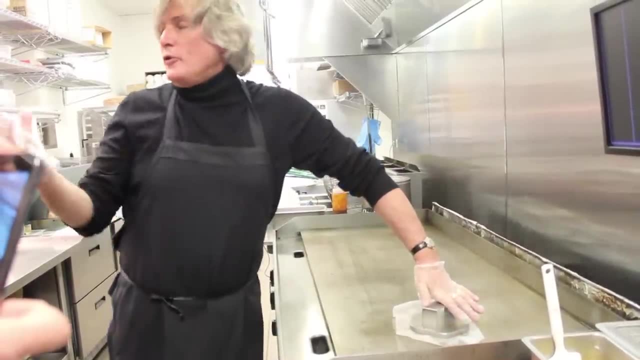 to meet the size of that burger. And the smashing technique is 10 seconds straight down metal to metal. And if you count, great, If not, there's a little timer here. What I'm doing, guys, I'm caramelizing the bottom of that burger, developing a lot of flavor, But I'm 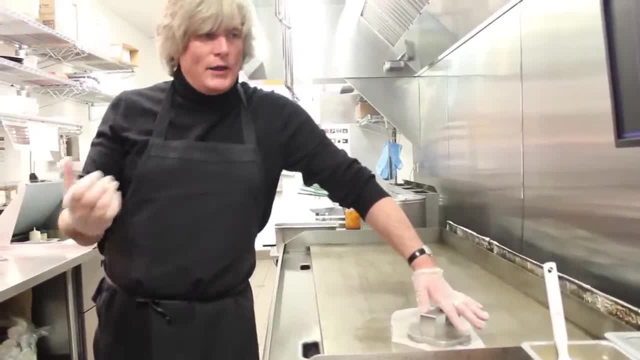 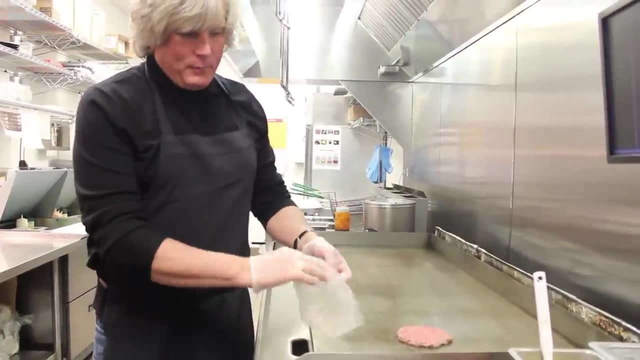 also setting up the texture and I'm also forming a shell, And why that's important is going to become obvious in just a second. The shell on the bottom of that burger is going to prevent that burger from cooking out. The juices are actually going to cook up. So if you notice, 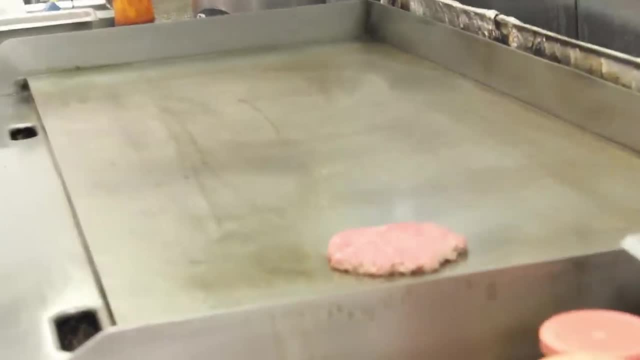 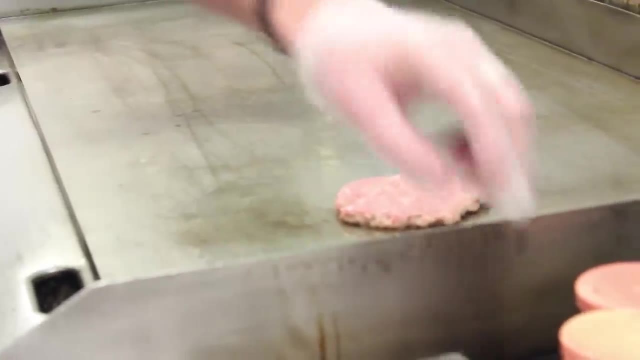 while you're eating the burgers tonight, you can probably taste the burger in every bite. That was the goal: Create a burger that cooks very quickly and uniformly that you can taste in every bite, And so I always tell people that one of the key things that this process lets us do is: 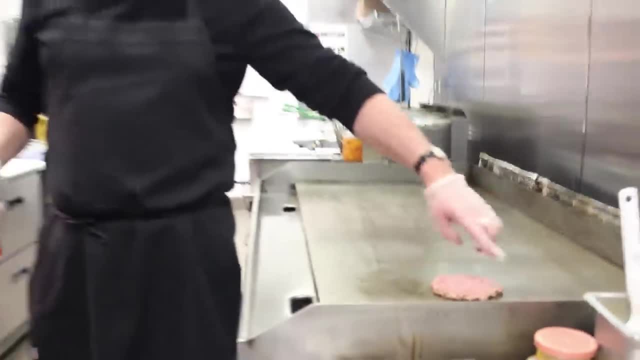 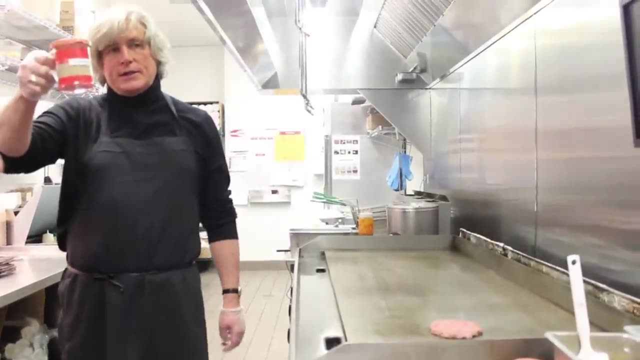 our burgers actually cook more like pancakes than burgers. You're going to notice that not a lot of the fat cooks out. You're going to see the juices start to percolate up through the burger. Seasoning is another important part of the smash burger flavoring Top secret. 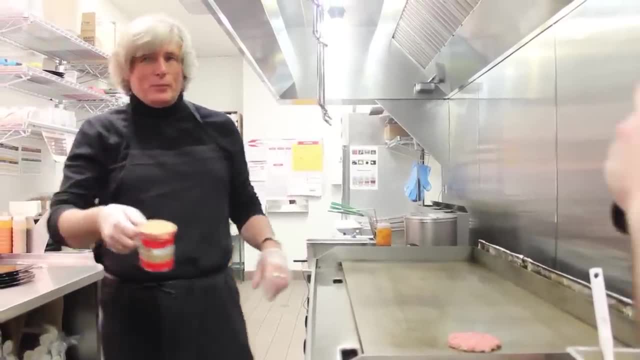 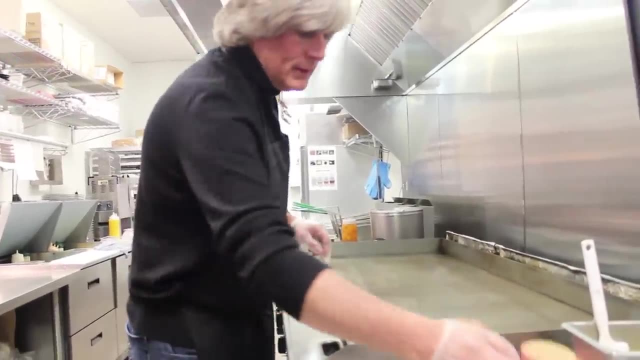 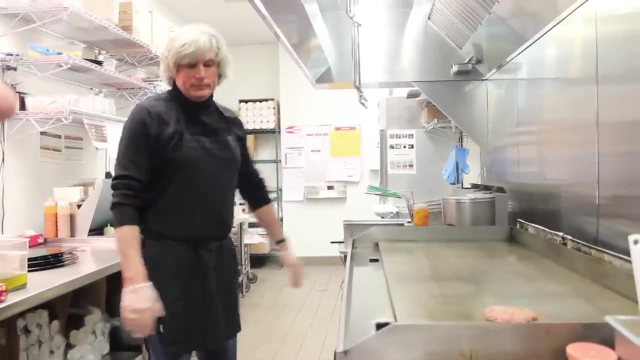 coat yourself with black pepper, garlic and a little bit of natural magic to bring out the taste of a certified Angus beef. So we season- if you're going to do this outside the air, And we cook these big burgers in about. I'll call it two minutes and thirty-five seconds. 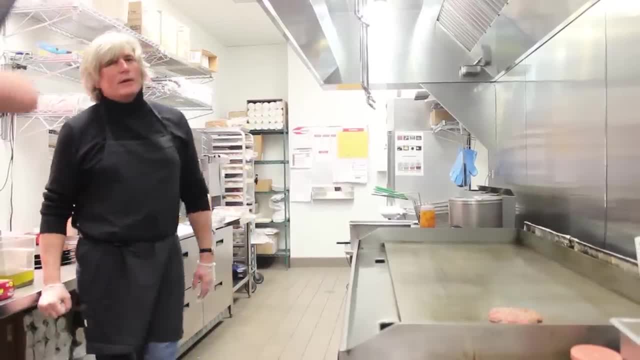 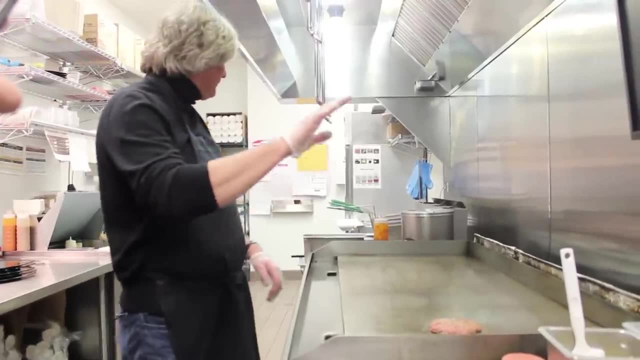 Hey guys, Guys, Here they come. Okay, They're special. Yeah, that'd be good. Oh, do you know where it is? I think I cleaned it. They cleaned it. No, I'm sorry, Tom, it's right there under your left side, under the grill. 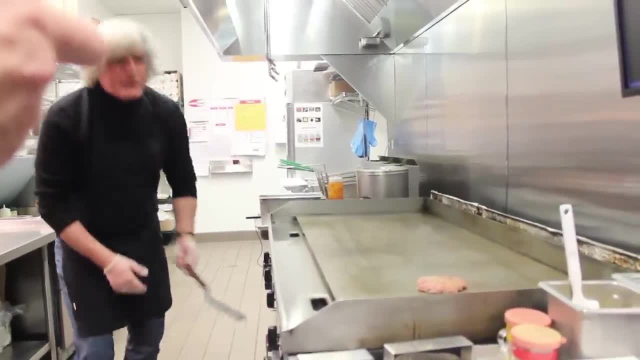 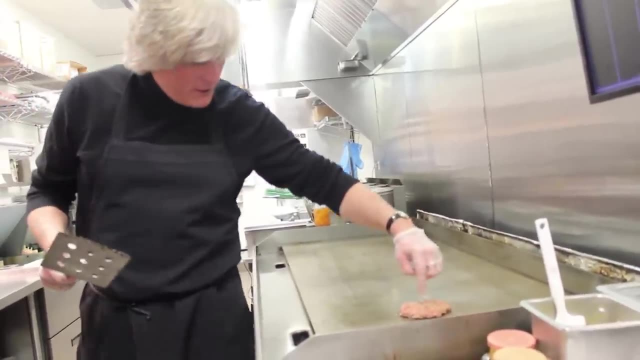 Here. Yeah, Oh, there it is. I'm sorry I didn't see it, Don't worry. So what's really important about a smash burger is: I've seared that bottom. I've seared that bottom. You start to see some of the juices cooking up through these channels. That's really an 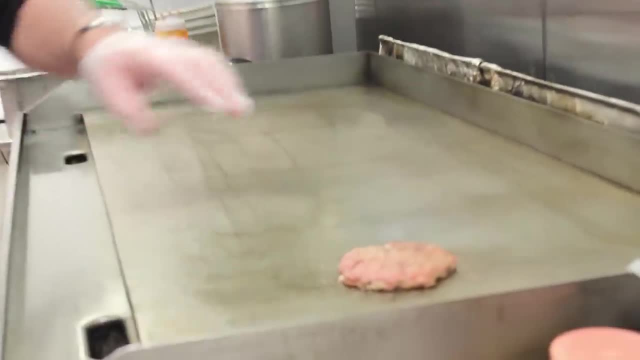 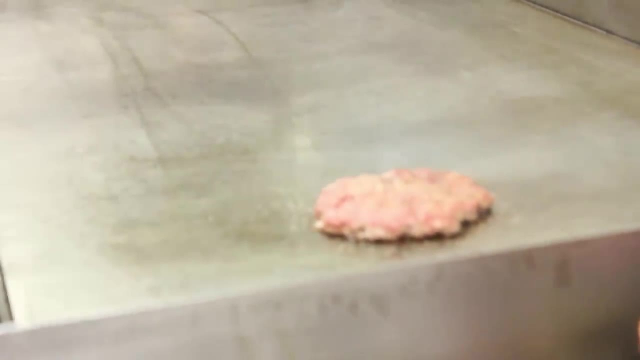 important part of what makes a smash burger a smash burger. But if I don't get that layer to come off with the burger, then I've kind of lost. So this is a very important part. So everybody who's going to cook a burger- you three right or your left-